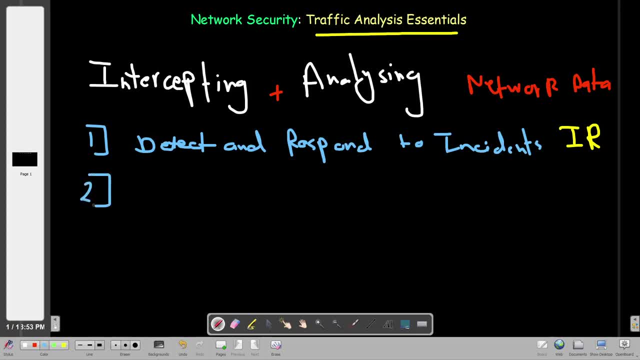 now, the other method or the other purpose of analyzing traffic is to troubleshoot network problems. so what do we do, basically, when we capture, when we have a packet capture, okay, we look into the data, we look into the protocols, the exchange packets. we have visibility on what's going on, what was going on in the networks, thus being able to analyze what. 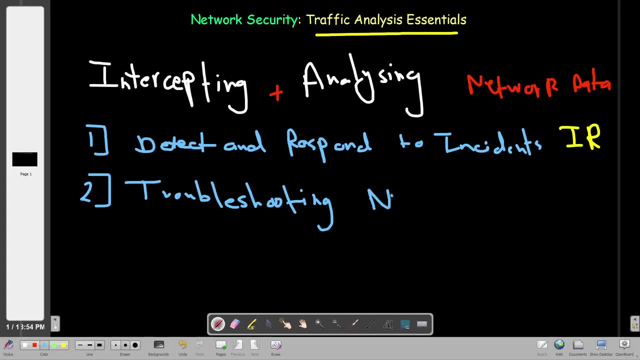 went wrong. so troubleshooting network errors, these are the two most common use cases for traffic analysis. so the first use case can be put under the security analysis. the second use case can be categorized or put under uh, network administration or network ни engineering. so basically we're interested only in troubleshooting. 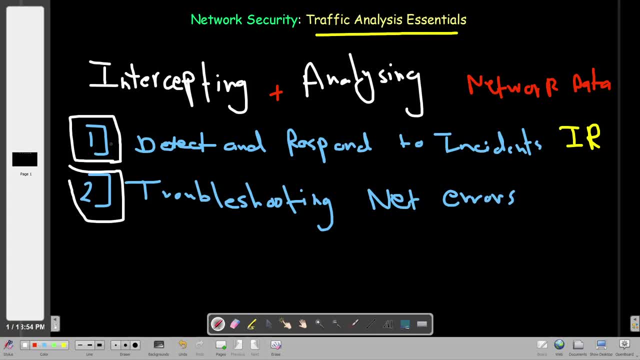 network errors, facing network problems, but, on the other hand, the first objective of traffic analysis is more concerned towards analyzing security issues or security incidents. so, okay, now let's talk about in details about, let's talk details about traffic analysis. so, basically, we said earlier that traffic analysis is part of network security and there are many things that can be. 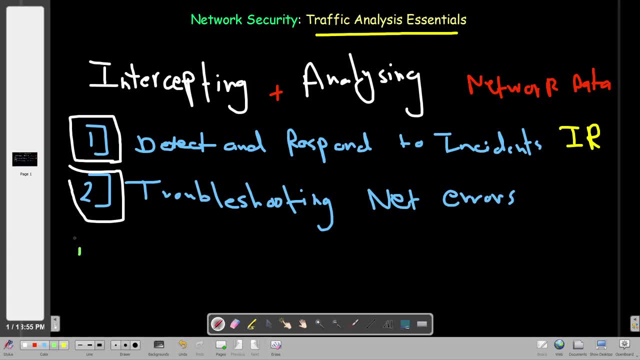 categorized or can be put under traffic analysis. so basically the first thing is network sniffing, net sniffing, net means network, so network sniffing, so network sniffing, is the process of intercepting network traffic and exporting the intercepted traffic into a pcaf file. this pcaf file, so basically we export. 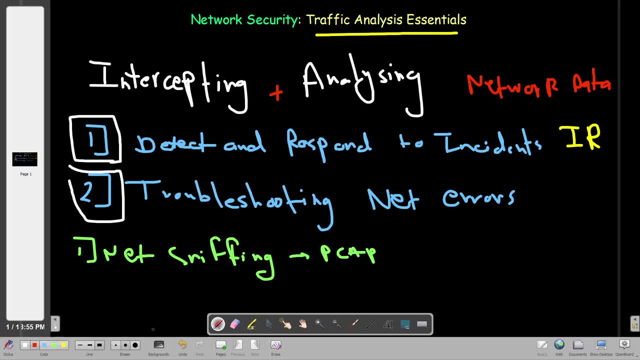 into a pcaf file and then this pcaf file can be opened using network analysis tools. so network monitoring is a very common tool for network monitoring, such as wire shark. another tool we discussed previously is bream. another tool was network miner. so now the next aspect is network monitoring: network monitoring, so traffic. 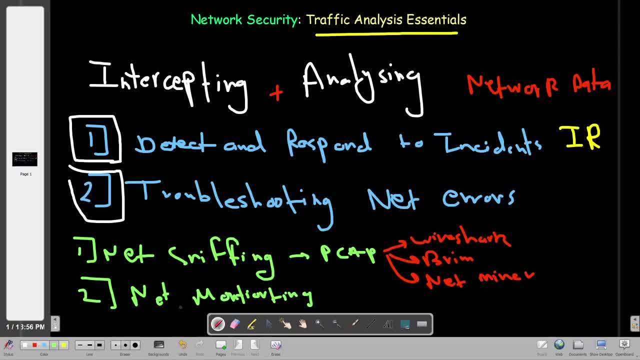 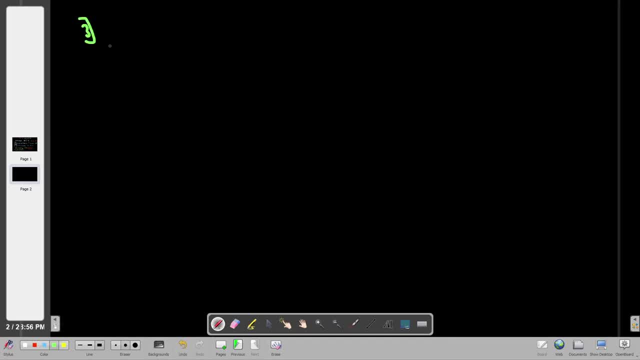 analysis. one aspect of traffic analysis is network monitoring page. now the third aspect of traffic analysis is intrusion detection and response, IPS ideas, basically all ideas or all IPS. we take the perform traffic analysis and pays on the traffic analysis and the configured rules. they trigger alerts, for example- let's take an example- snort. snort is an ideas. 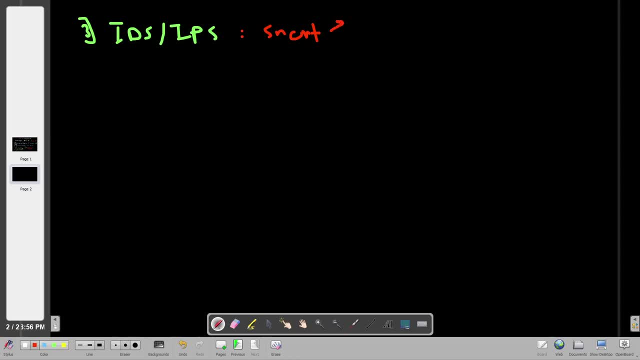 intrusion detection system after configuring snorts with rules- okay- and alarms. what's going to happen here? snorts will analyze the traffic. based on the analysis, it will trigger alerts- okay, based on the traffic analyze- and, of course, the rules. another aspect of network analysis, or traffic analysis, is 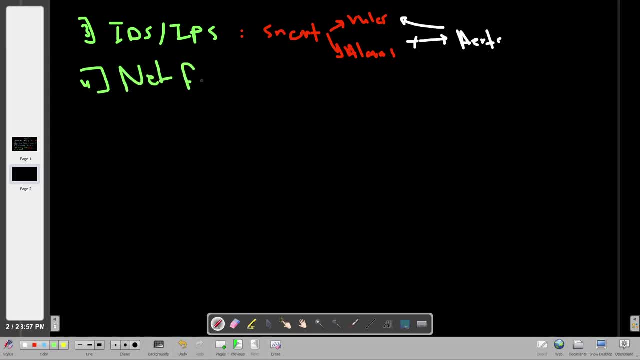 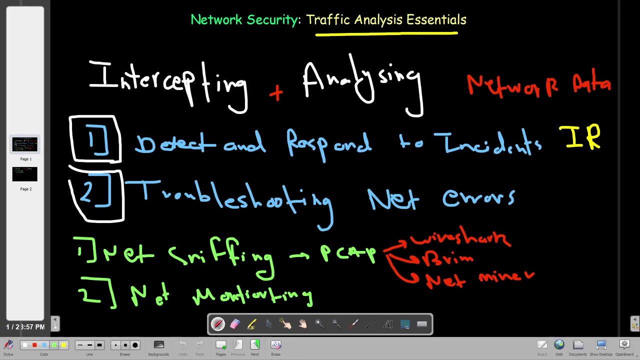 network forensics and the last aspect is threat hunting. so all of these aspects, the things we mentioned here, and in addition to network sniffing and monitoring, can all be aspects of traffic analysis, can all be things you do when you analyze traffic. so let's now discuss the two main techniques in traffic analysis. so 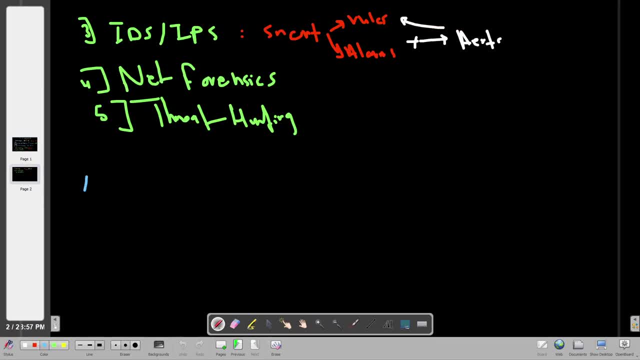 we have two main techniques in traffic analysis and the first one is the traffic analysis and the second one is the flow analysis. so we have two main techniques in traffic analysis, theoretically. so traffic analysis techniques, we have two. the first one is, we call it the flow analysis- flow. 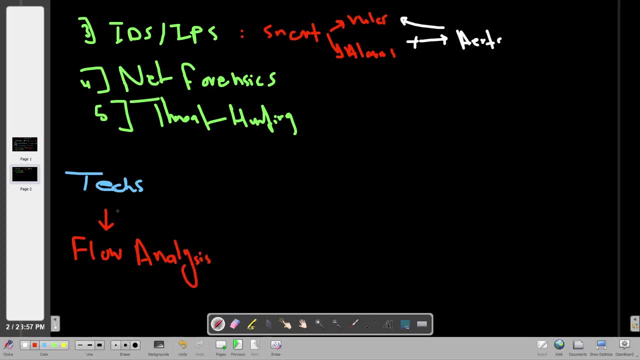 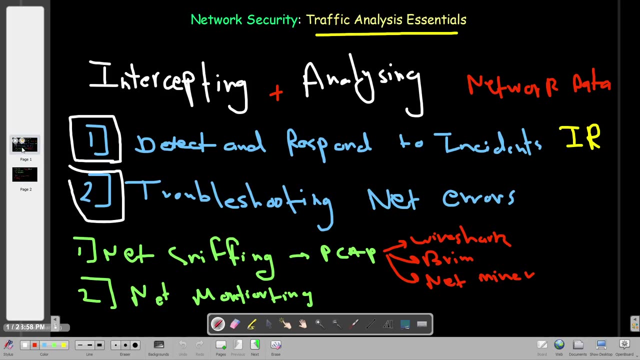 analysis. the other one is packet analysis. okay, so what do you mean by that? when we answer or when we not, we talk about the techniques, so we will stand from where the network data is coming. so, basically, we have said earlier that we are concerned or we want to, uh, in traffic analysis, we want to analyze the network data, right, so 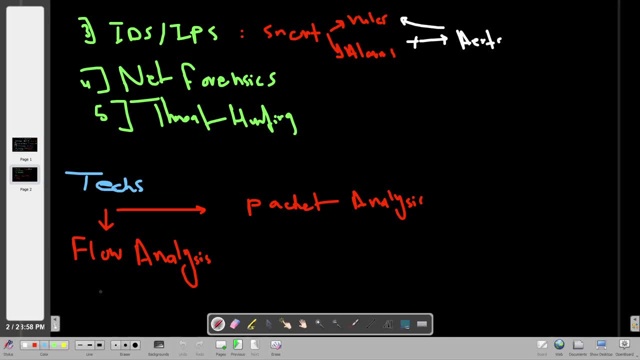 network data comes from network devices. so in flow analysis, what we do here, we only go through the statistics, the stats about the network. so how do we read these statistics? these statistics can be read directly from the network device. so what are the network devices? switches, routers, firewalls. 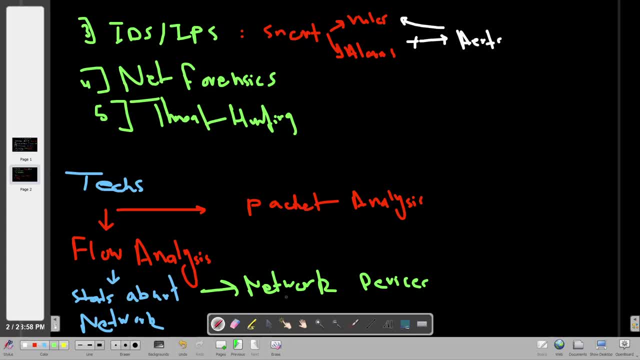 other appliances that configured in in the network, all of these appliances you can inspect the traffic directly from directly, by looking into the appliance interface and then looking at the logs, looking at the live traffic. so based on that you can perform flow analysis. so in flow analysis we want to look at the statistics. so statistics. 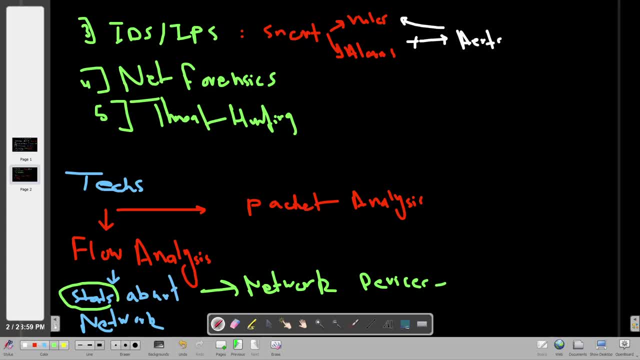 mainly come from network devices from which you can create dashboards. so when you read the dashboard of a new device like router or firewall, you can have a brief overview of the statistics about the network. we call this flow analysis now packet analysis. in packet analysis we perform the 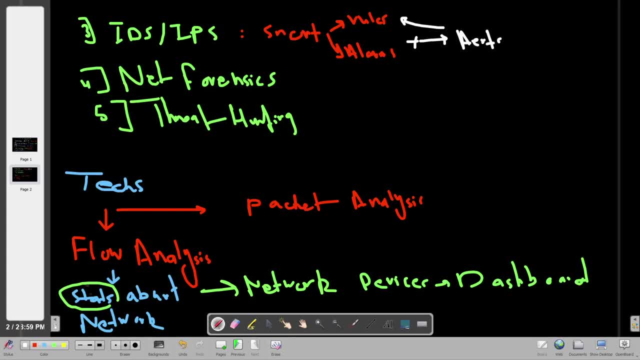 detailed analysis of the packets. we not only go through the statistics. what we do, yeah, we pull, we pull the statistics, but at the same time we want to uh, pull the logs. okay, or let me remove this one- pulling the logs into pk file, and then the pick up file can be exported or can be downloaded. 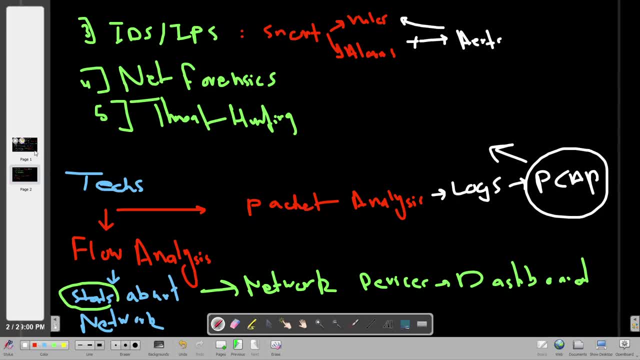 directly from the network device. okay, into the network device. so the network device can be exported to any traffic and or network analysis tools such as wireshark, brim or network miner. that's how the flow works. so two techniques of traffic analysis: packet analysis and flow analysis. okay, and now? 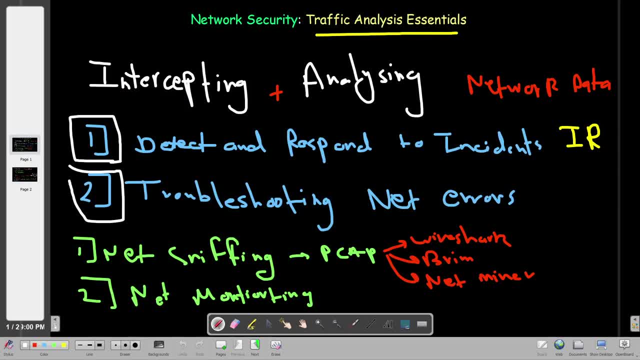 let's go back a bit to see what we have achieved so far. so we talked about traffic analysis, with defined traffic analysis. we talked about the two main or two common objectives of track traffic analysis, which are detecting and responding to incidents and troubleshooting network errors. also talk about some aspects of traffic analysis like network sniffing, monitoring, troubleshooting. 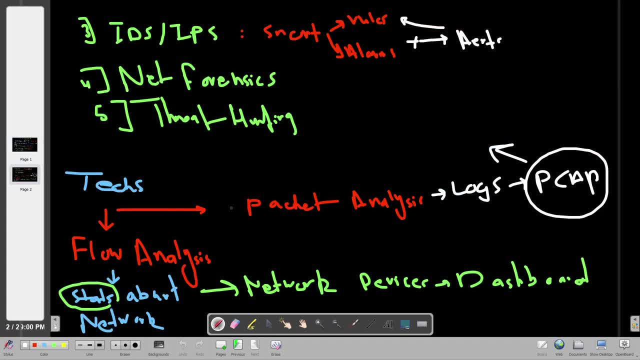 and lastly, we talk about how to perform traffic analysis. so basically, we can directly export the logs from the network device into a pickup file- we call this packet analysis- or we can log into the user interface of the network device and look at the dashboard and statistics. to briefly uh, 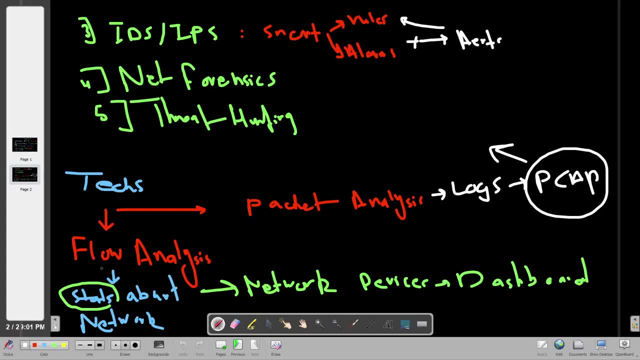 you know, find out what's going on in terms of numbers. okay, so now we will take an example. okay, and perform packet analysis. okay, oh, sorry, not packet analysis, it's going to flow, we're going to perform flow analysis. so the flow analysis we perform now is part of a room into a hack, me called. 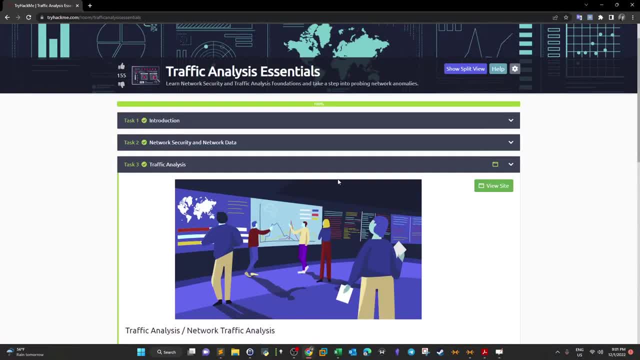 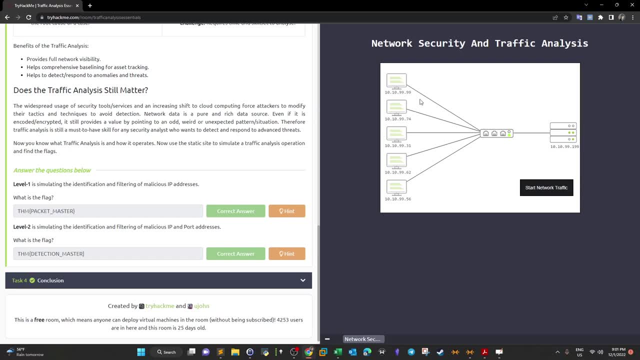 traffic analysis essentials. so we have a challenge in here. we're going to open, we're going to click on a view site and we take a look at the challenge. so, as you can see, here we have a topology. as you can see, we have a couple of pcs. okay, these pcs, they exchange traffic with. 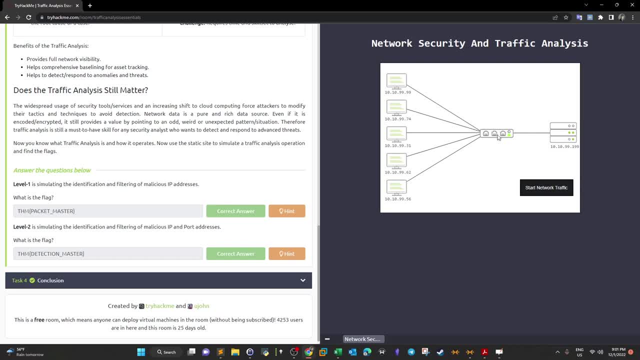 this switch and then they send the traffic to the switch and from the switch to the- as you can see the router here. so we want to find out if there is malicious traffic coming from one or some of the pcs in here. so this is only simulation of traffic analysis, right? so basically, what we do, mainly we, only we can. 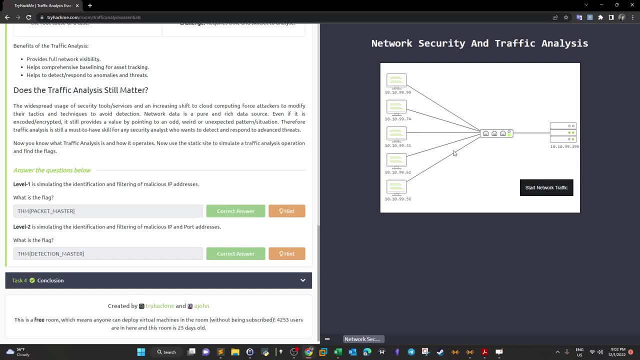 either record the traffic in here and take it into pickup file. we can directly from the firewall. you can take this as a simulation of directly analyzing traffic from the network device. it's going to start network, start network traffic, as you can see. now the packets is coming from these. 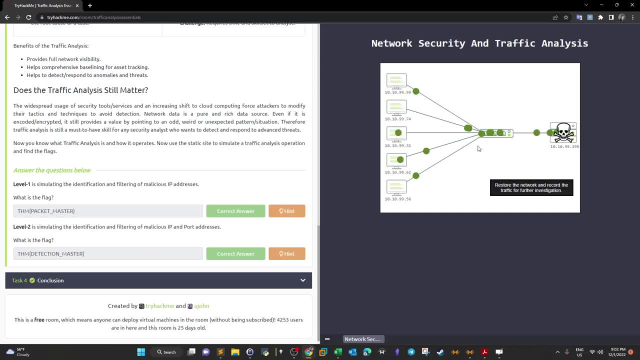 pcs- and we have red dots here- represent the malicious traffic, as you can see. now it's saying: restore the network and record the traffic to further for further investigation. right now the traffic is flowing right. what we want to do, we want to log these uh packets, okay, in order to analyze. 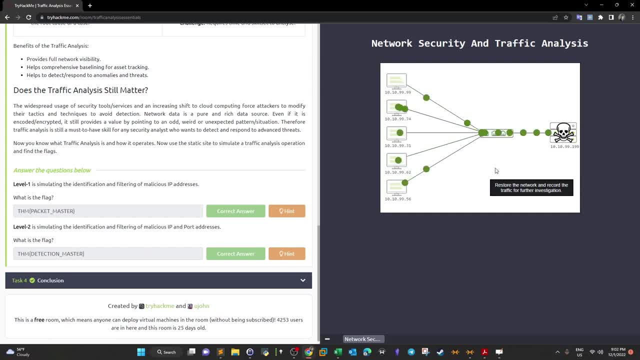 them in in packet analysis. we record and we export. so right now we're going to only record the traffic, because it's only a simulation. so right now it's gathering or it's recording the traffic. as you can see, it's creating a log file. normally this log file comes in a 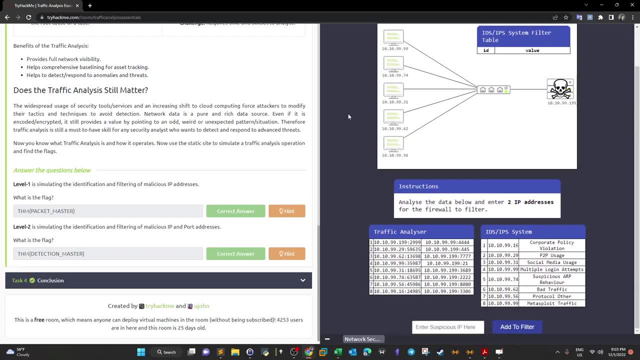 format. okay, so let's see now. what do we have here? so these are the statistics we talked about earlier that can be presented in the dashboard of the network device. so the instructions here we have: analyze the data below and enter two ip addresses for the firewall to filter. how to find out what 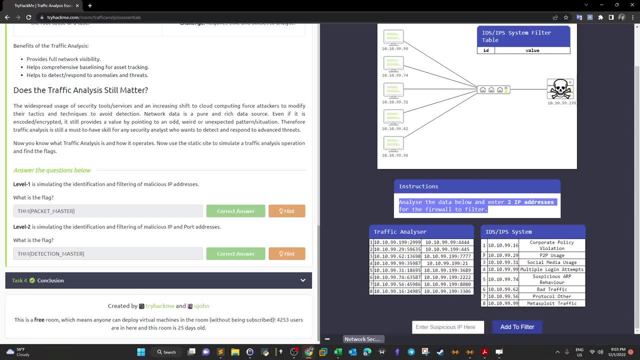 are the ip addresses that could represent a threat to the network. so we have here, as you can see, the different ip addresses in here from the traffic analyzer and we have the ips according to the ids ips. so basically, this, this table represents the different categories of the alerts that have been triggered, based on the rules configured in the ids. 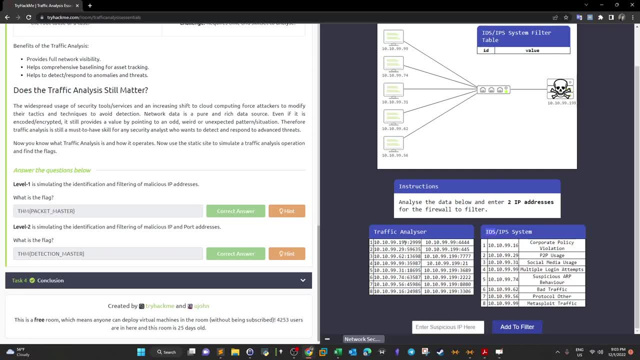 slash ips system. in here we have the traffic exchange between the pcs and what represents here, maybe the server. so basically, uh, of course, we have the port, the source port, destination, port, source- i'll be- destination ip, okay. so the first thing we want to look at is the um. 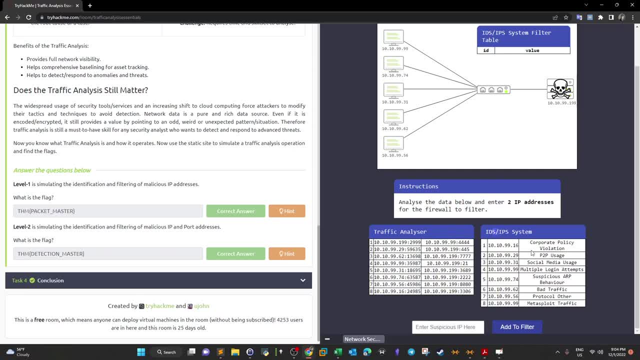 alerts that have been triggered by the ids. we have the categories here: corporate policy violation. we have p2p usage, social media, multiple logins, suspicious arp, bad traffic. so i know more than two of these may represent a threat on the network, but we have to narrow down our choices to only two of 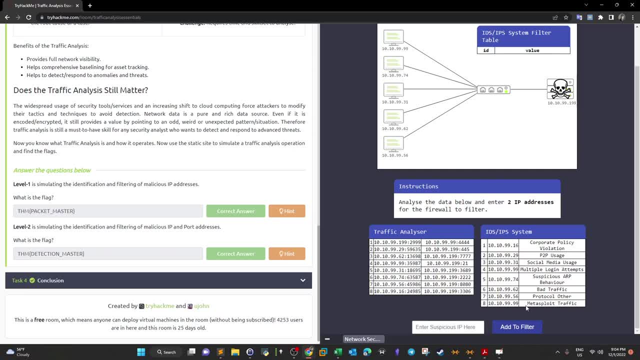 these uh categories. so, as you can see, we have metasploit traffic. this alert has been triggered by the ids and we have um bad traffic. multiple login attempts can also represent a threat to the network, since it since it may indicate that there is a brute force attempt. uh, also, we have suspicious rp heavier. someone might. 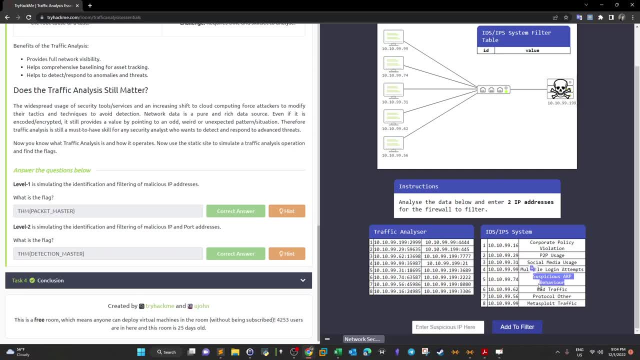 be intercepting traffic to perform man-in-the-middle attacks also. this represents threat on the network. corporate privacy violation may also present a threat on the network, since it may indicate that sensitive data is being carried uh off the local network, so this alert can be uh thrown. if this happens, corporate policy violation. okay, let's take a look at metasploit. 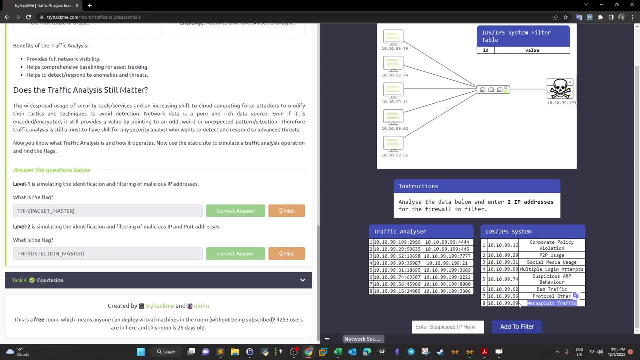 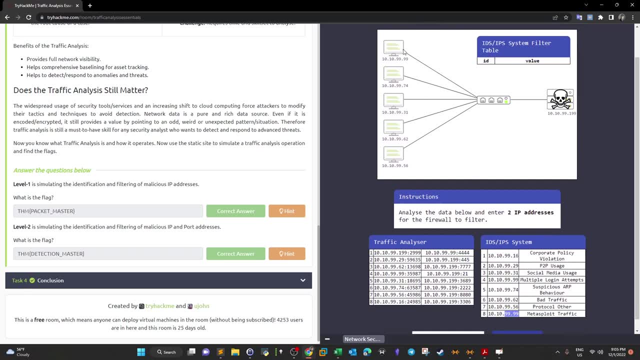 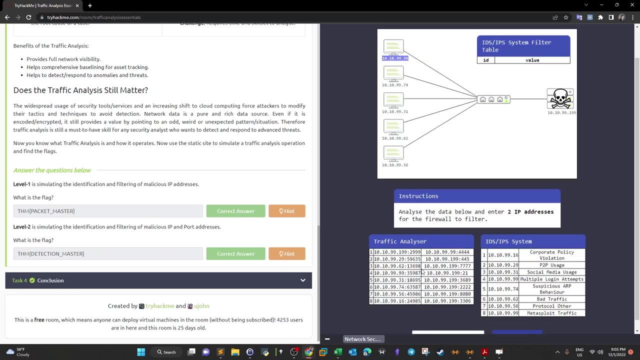 traffic. so, as you can see, metasploit traffic is, uh, coming from the ip that ends with 19, 9, sorry, 99, so 99. ip the pc that ends with us this ipsc here. okay, and that's the first ip address you want to filter. so we're going to copy the ip address and we paste here at the 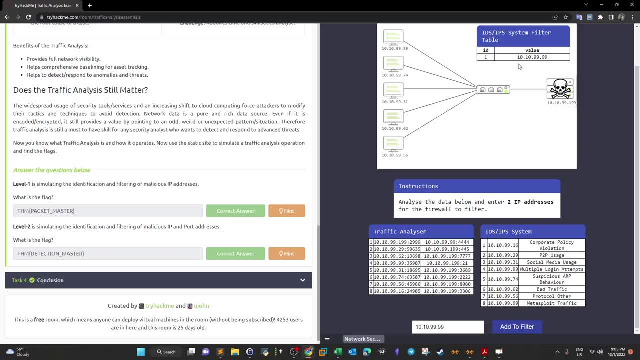 photo. so we've added the first ip address. next thing i want to uh look at the other ip address that may represent a real threat on the network. so multiple login attempts is a candidate. but in this scenario here the bad traffic is the second real threat on this network. so we're going to take the bad traffic as you can see it's coming from. 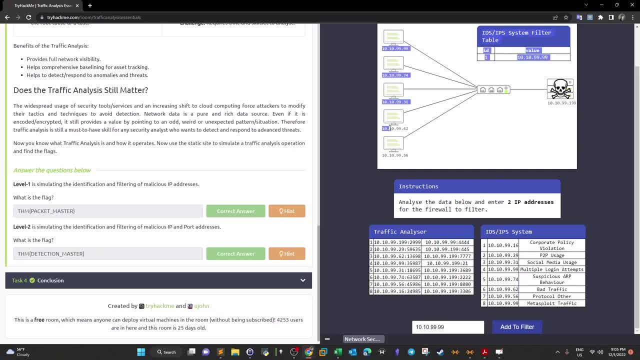 ip that ends with 62. it happens to be this pc and if you look at the traffic analyzer, if we take a look at the ip, as you can see, 62 right, the source port is 13 698 and the destination port is four sevens. 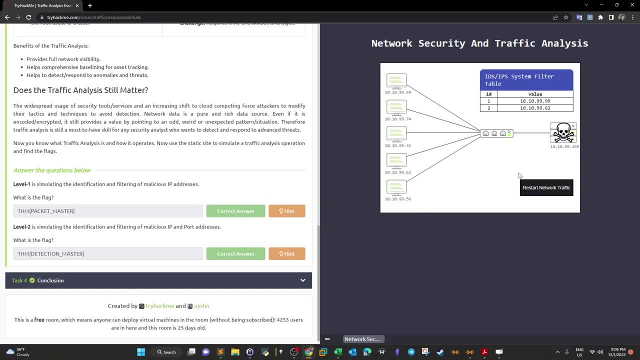 so we're going to paste in the next ip and then we're going to restart the network traffic. we're going to find out if the malicious traffic is blocked or not. we can. we can see that by monitoring the red dots that's coming from these devices, devices, if the red dots make it through to the 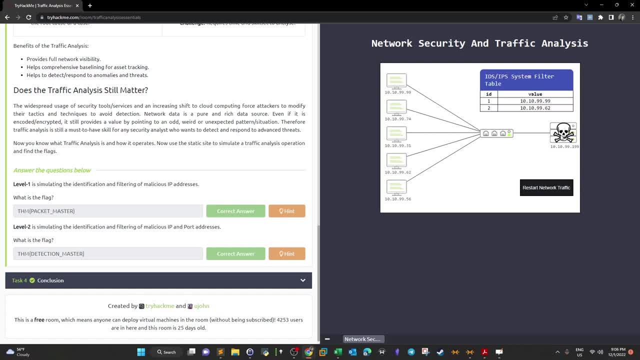 final destination. it means we have something wrong. if the red dots they don't make it through the switch. here, it means our work was correct. so restart the network traffic and let's monitor the red dots. let's see here: as you can see, the red dots did not come through this. 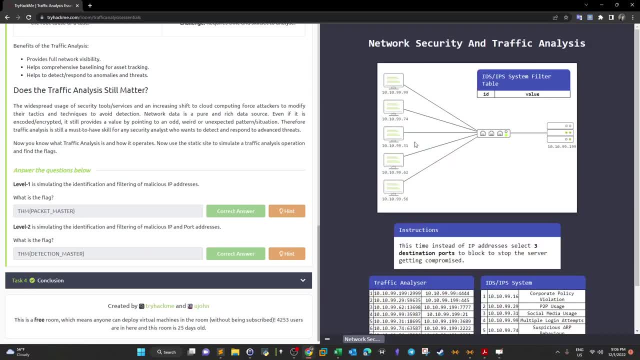 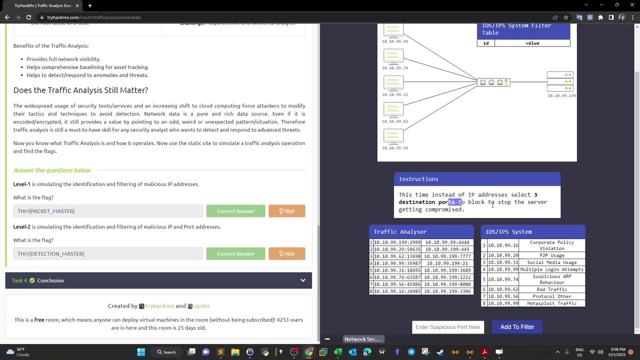 so this one is correct and that's the flag for the first question. now we have the next task. this time, instead of ip addresses, select three destination ports to block to stop the server getting compromised. so, again, in addition to blocking ip addresses. okay, as you can see now. 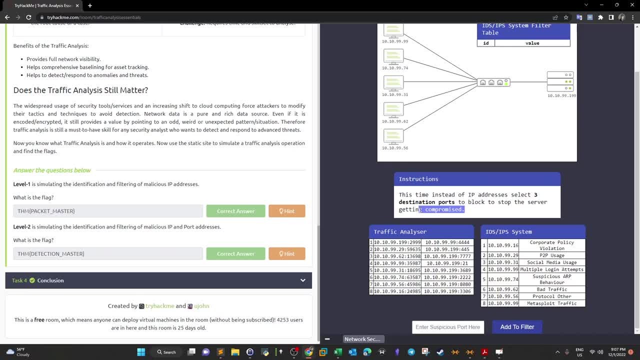 we are practicing, or practicing, as you can see, the first objective of traffic analysis: responding to threats. so, analyze the traffic. we found two malicious ip addresses. we added them to the firewall to block them. that's how reality works. now, in addition to blocking ip addresses, as you can see here, we're gonna block the ports. so let's go back to the v мет sentence. here we can block the doors. so we're going to see, we're going to be able to realize that there's not only access to theasses like this, but we also might use the red dots instead of connecting, which is we're going to side by side. now we can see that our dataここ slash address, the address. we're going to see. 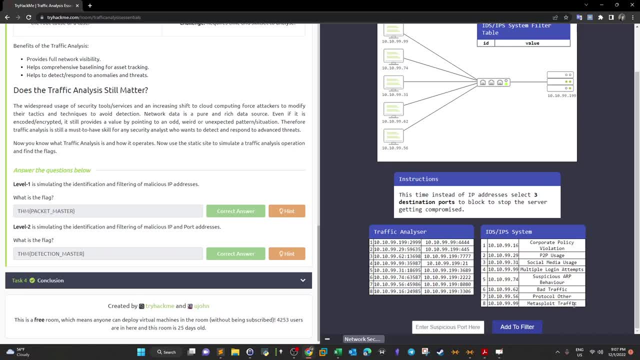 to block the shifts, we get to virtual and if you have styles like this and, as you can see, using thealed, let's go back to the table here and remember what's where, the categories that trigger the alerts. so we have meta supply traffic and also bad traffic. let's go to the corresponding ip address. 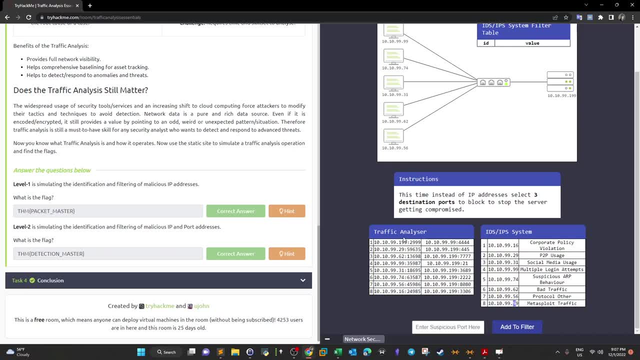 here it's the ip that ends with 99. if we go to the traffic analysis table here and look through the table, we can see this is the ip address here and this is the destination port: it's 21.. so we're going to have to block the 21 port. 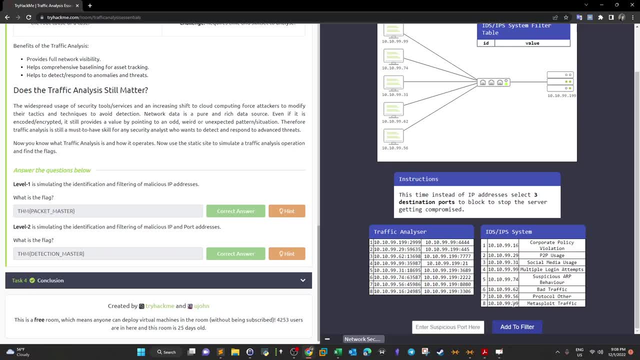 that represents the ftp traffic. is that correct? let me see, do we have 99, 10, 10, 99? so the first port is 21, which is weird. it means that the ftp server will be blocked from this ip address. they will be blocked from accessing the ftp server. and next ip was: 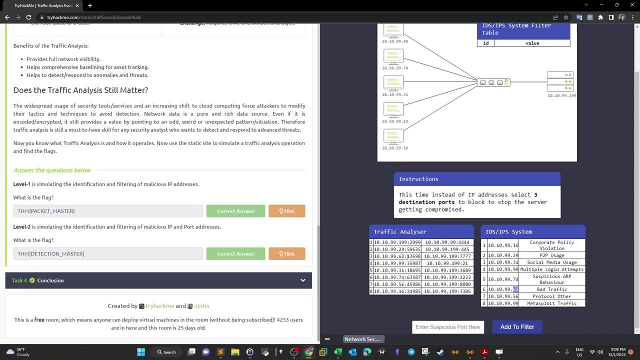 that the one that ends with 62. it means we're going to block port 13, 698. so we're going to take this. so thus far we have three ports, we want three ports, that's why we have two. so we have 21 and we have seven, four, sevens. 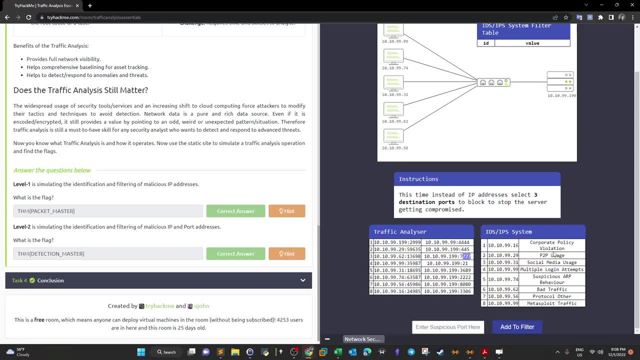 okay. so let's first block the first port, ip, that ends with 62, four sevens. i'm not sure about the port 21, because it represents a real service, so we're gonna block four sevens here. okay, now let's take a look at the other ports. so we have port. 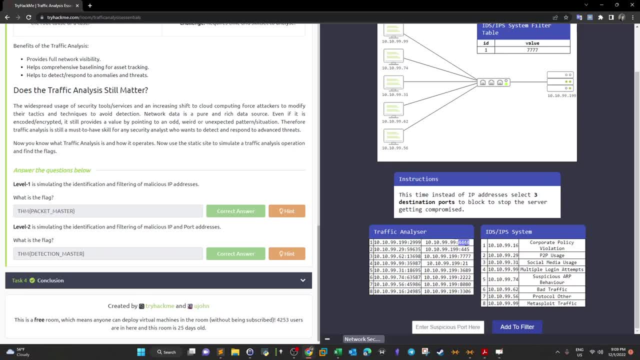 444's, as you can see here. yeah, so most probably this is the port that we need to block, not 21, right, because 21 represents the ftp service. 21 represents the ftp service. 21 represents the ftp service to be server. we're not going to block a public service, right? so we're going to block this ip. 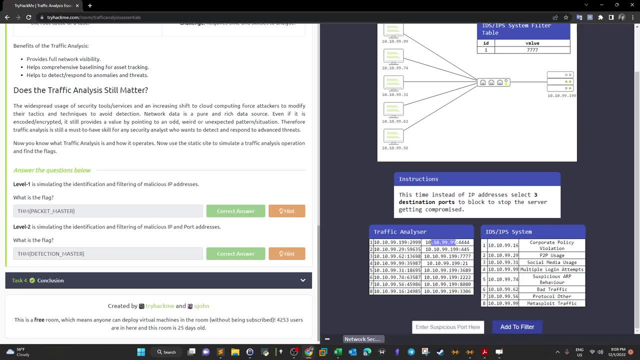 at this port. it corresponds to the ip address from which the meta split traffic has been witnessed and it happens to be destination port. so we're going to block this port. so we have two now the rest, we have three ports. we blocked the meta split traffic, we blocked the. 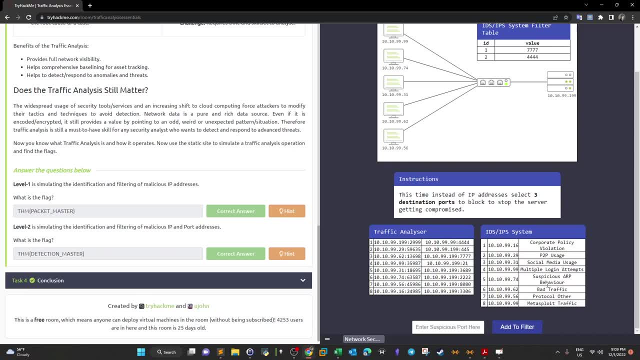 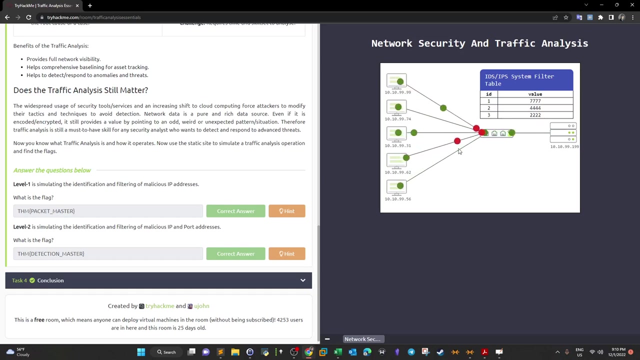 bat traffic 62 and, as you can see, we have suspicious r behavior. ip 74. as you can see, the station port is two tools. uh, four, two, sorry, let's see. let's monitor the red dots. will they come through? nope, as you can see, it worked. so that's it, guys.